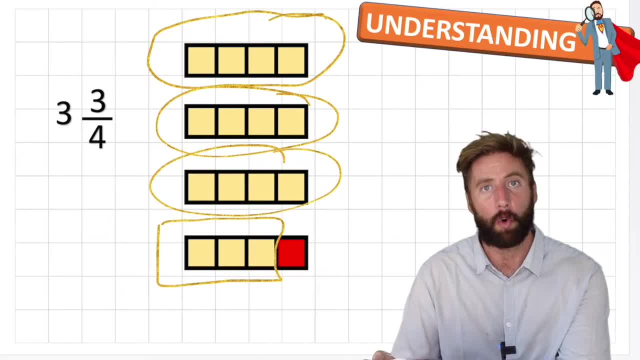 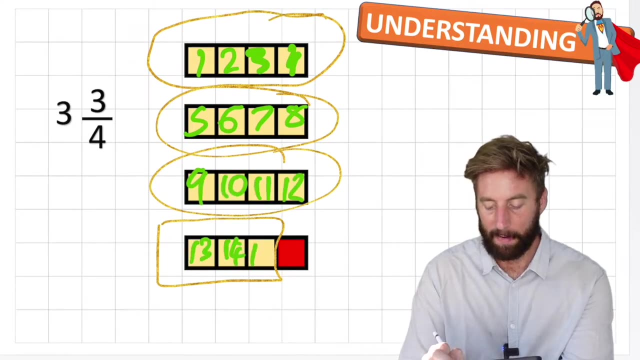 So then, improper fraction is basically asking: how many quarters do you have, but without the mixed number. So we can see here that we have one, two, three, four, five, six, seven, eight, nine, ten, eleven, twelve, thirteen, fourteen and fifteen. 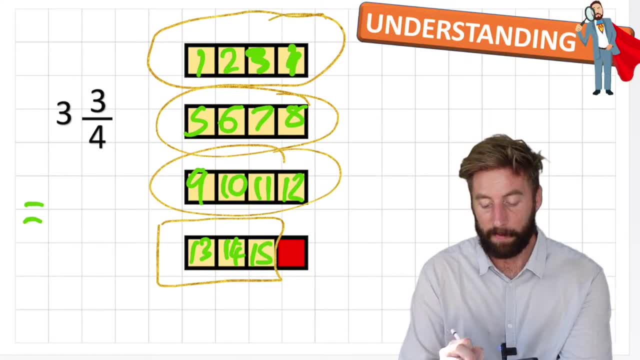 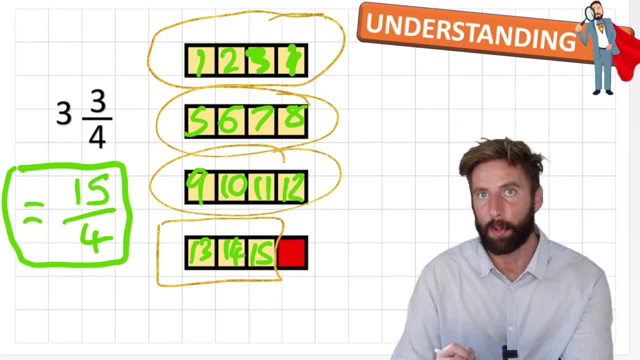 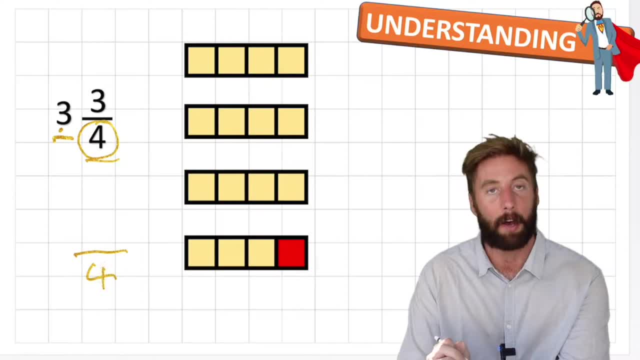 So we know we're going to have something- quarters- as our improper fraction, And the way that we can find out how many quarters we're going to have is we can simply times our four by our three. And the reason that is is because, look, we have three whole, two and three. 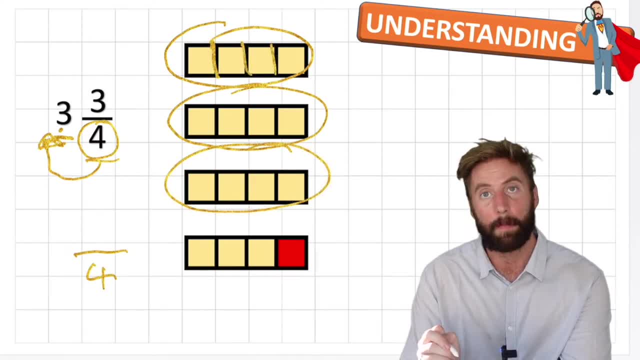 Each of these wholes is split into four. So therefore, if I times, If I times three times four, it's going to give me how many quarters I have in my whole number. So the answer to three times four is twelve. But I'm not finished yet, because of this last three here. 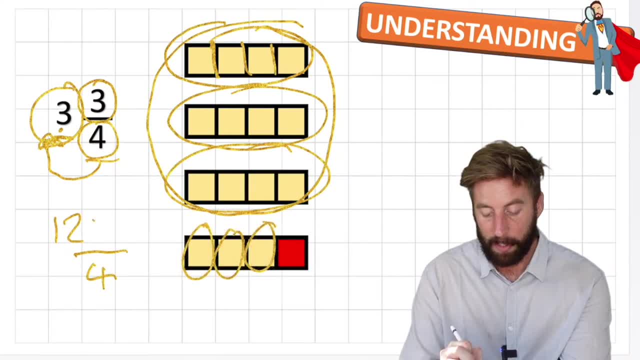 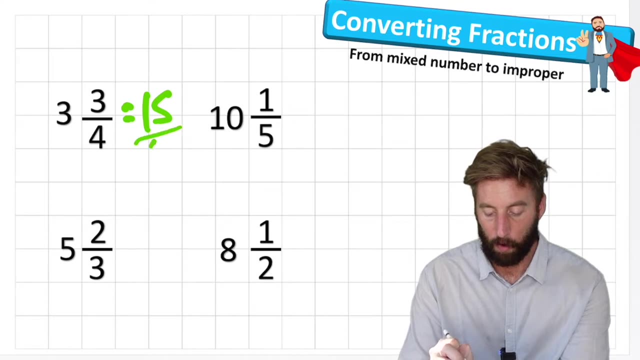 Now this is just three on its own: one, two, three. So therefore I need to plus three. So my fraction is twelve plus three fourths. Therefore it's going to be fifteen fourths. Okay, so the answer to question one is fifteen fourths. 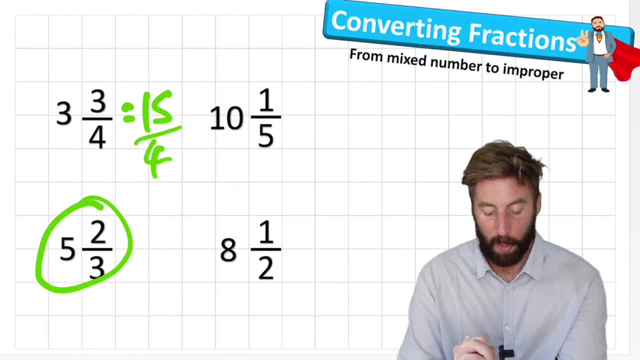 Okay, let's have a look at the question one. Question two: let's have a look at five and two thirds. So five and two thirds. Well, let's not bother building those bar models again, Let's go simply into the method. 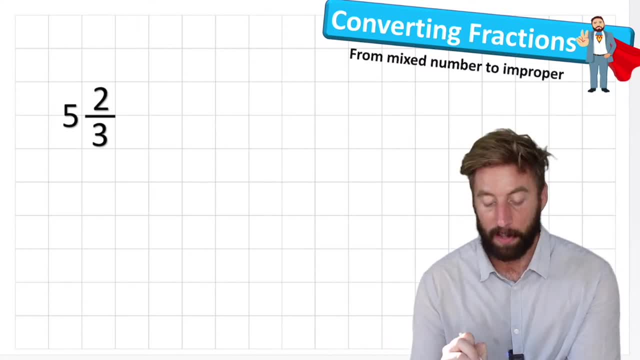 So the first question I want to ask myself is: what is my fraction? And in this case it's third. So I know that my answer is going to be in thirds, for the improper fraction, How many thirds do we have? Well, let's find out. 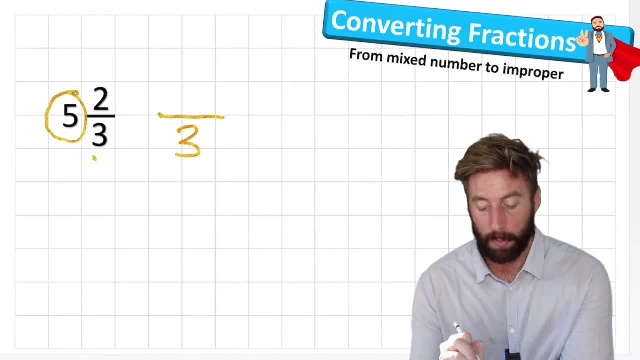 How many thirds do I have in my whole? I know now that I can just times three by five, and three times five equals fifteen. So I have fifteen. But remember, I'm not done, because I've got this pesky little two here and that was just. 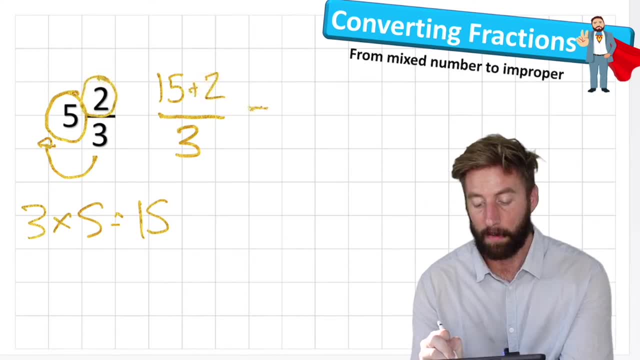 going to be added on. So fifteen plus two. Therefore, the answer is seventeen thirds. So the answer to five and two thirds is seventeen thirds as an improper fraction. Now, before we move on, let's just make sure that's right by flicking it back to a mixed 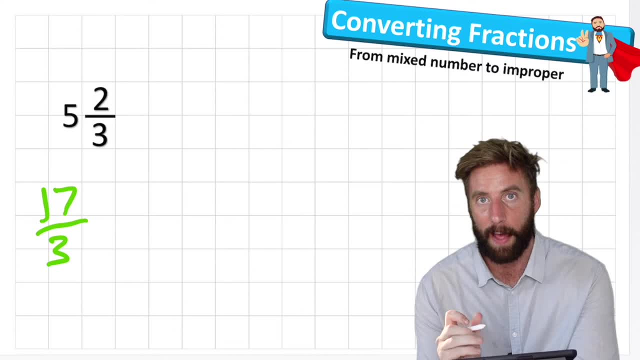 number in the way that we learned in the previous lesson. So if you haven't learned that, go back and check that out as well. So we're going to turn it back into a mixed number by simply dividing seventeen by three, Because, if you think about it, division is the inverse of multiplication. 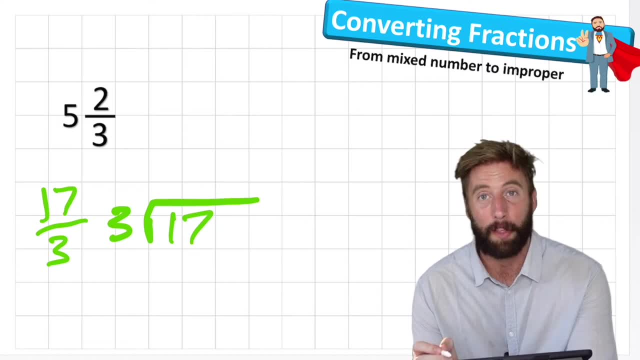 So we're going to obviously divide at this point if we're trying to find the opposite. So how many threes are there in seventeen? Well, there's five, remainder two. So therefore my question: so therefore, my mixed number is going to be five and two thirds. 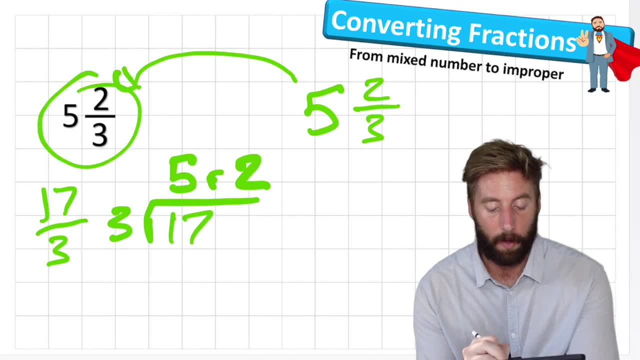 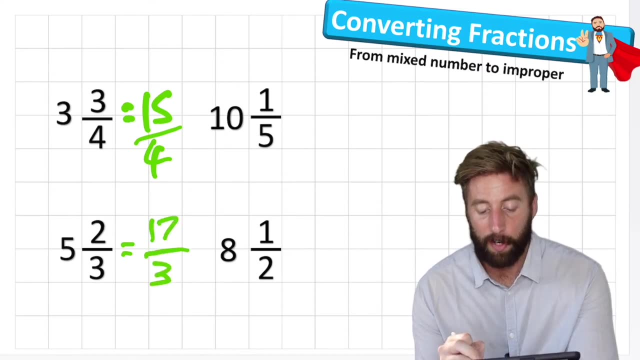 Is that correct? Yes, it is. So we know this is right. So five and two thirds is seventeen thirds- Awesome, Okay, let's look at question three. ten and one fifth. So ten and one fifth. let's do this really quickly now. 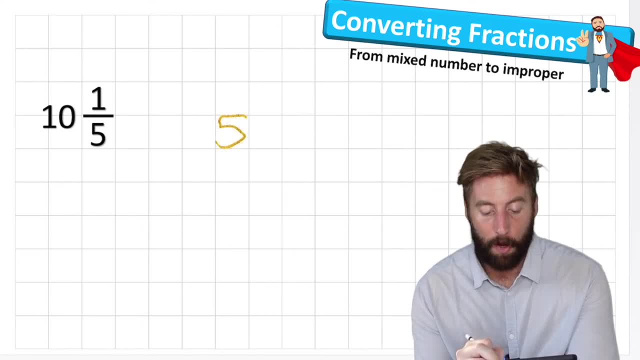 So what we can do, we know we're going to be working in fifths And we know that we can multiply our five times ten. It's going to be fifty plus the one is fifty one. So I've got fifty one fifths. 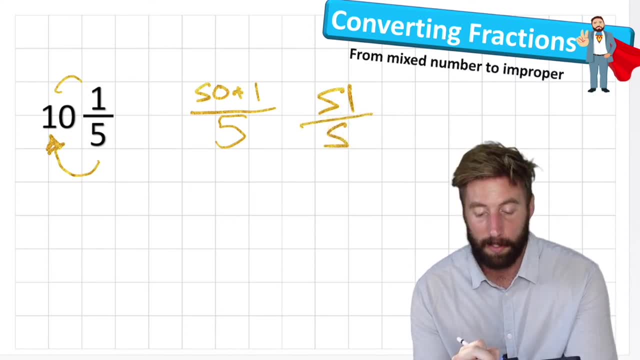 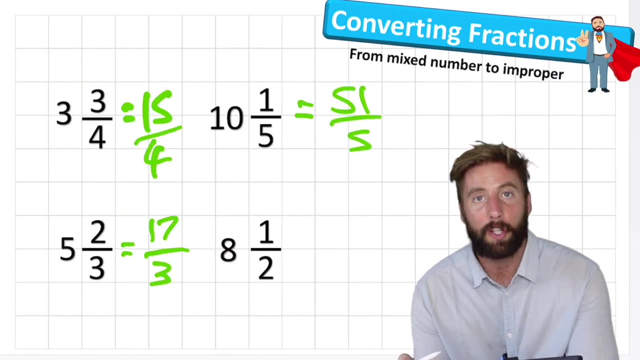 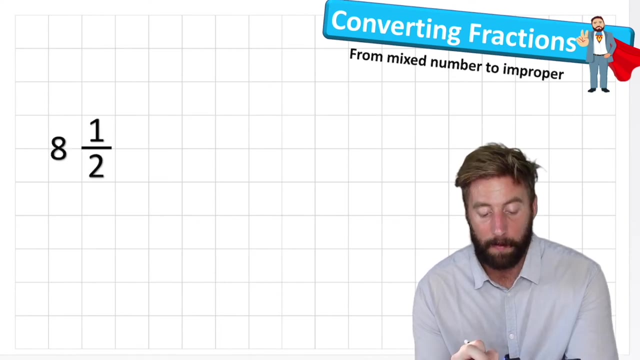 Huge improper fraction there. So my answer to ten and one fifths is fifty one. I'm going to give myself a tick for that question. Okay, final question, and we're going to look at question four. eight and one half, And the question is asking me: how many halves do I have? so I know that, therefore, I'm going. 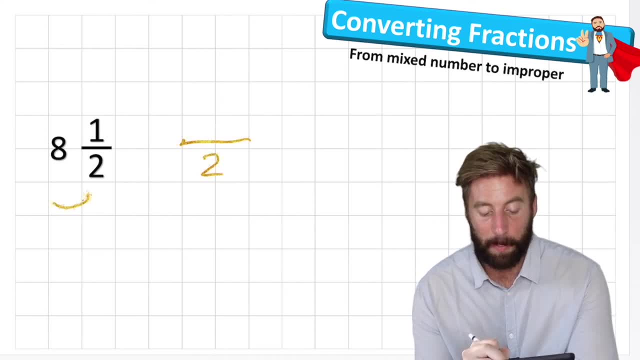 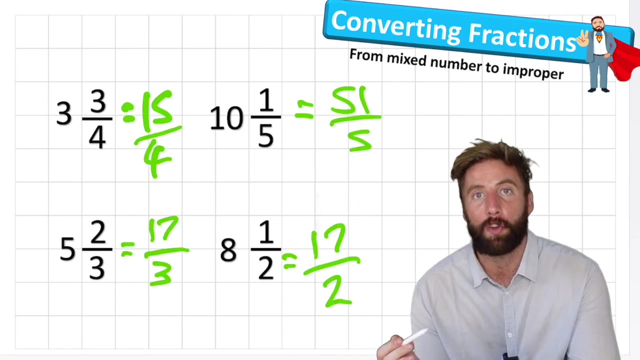 to have halves as my denominator, And let's just simply times eight times two is sixteen plus my one is seventeen, So I have seventeen twos. Super quick: One One, Two, Three, Four, Five, Six, Seven, Eight.